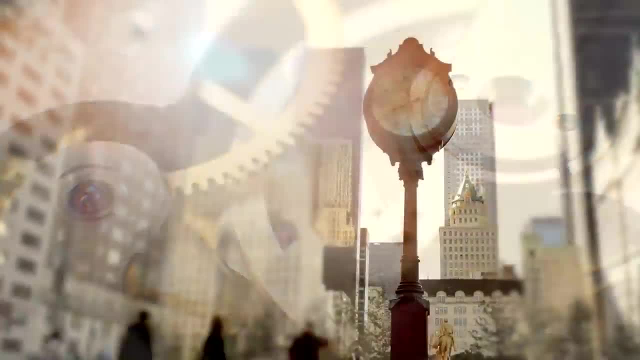 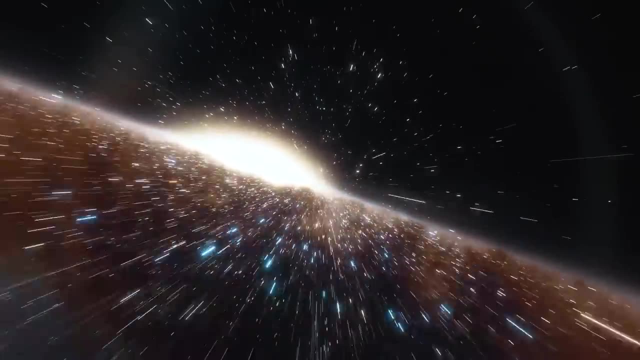 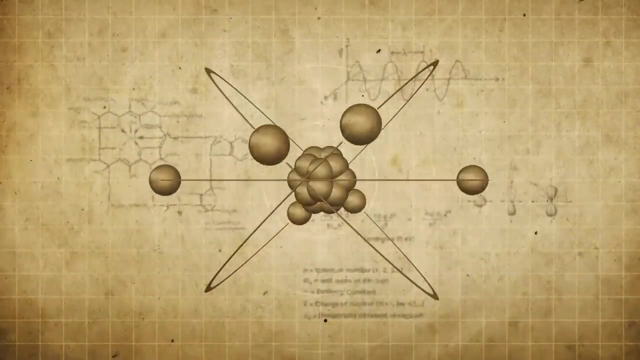 It would be a mechanical clockwork universe where everything was predictable and deterministic In principle. if we had all the positions and velocities of all particles in the universe, we could predict the entire future of the universe as well as precisely know the past. This was the way the universe was thought to be about a hundred years ago. 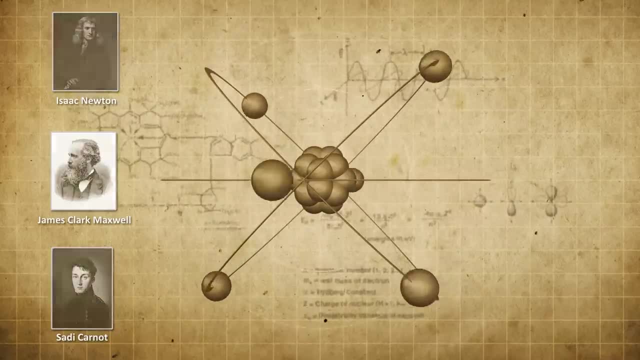 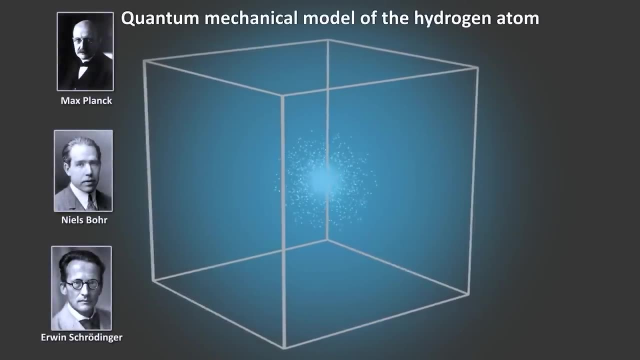 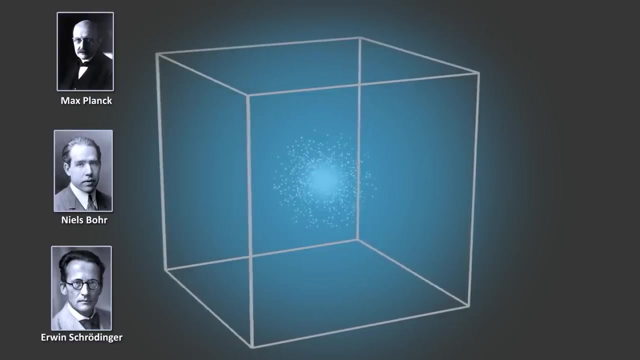 It was a classical picture of the universe, defined by classical physics. Then quantum mechanics came along and poured cold water over this idea. This changed our view of everything. At the most fundamental level and the tiniest scales, reality turns out to be probabilistic. 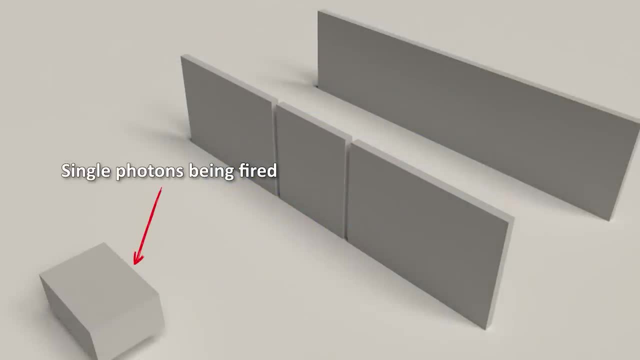 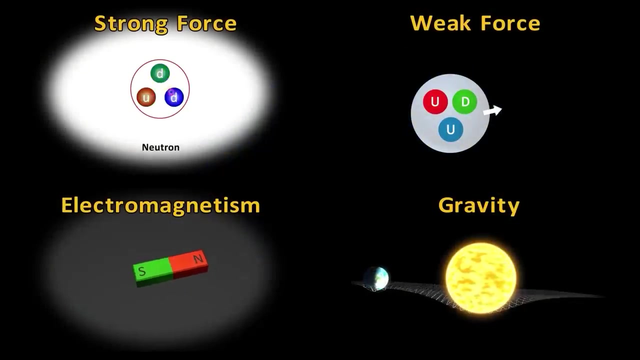 The precise location of a particular particle cannot be predicted in advance, even in principle. Yet this idea, as defined by the rules of quantum mechanics, is the best and most accurate theory we have about the way the universe really works. It can account for all the forces of nature except gravity. 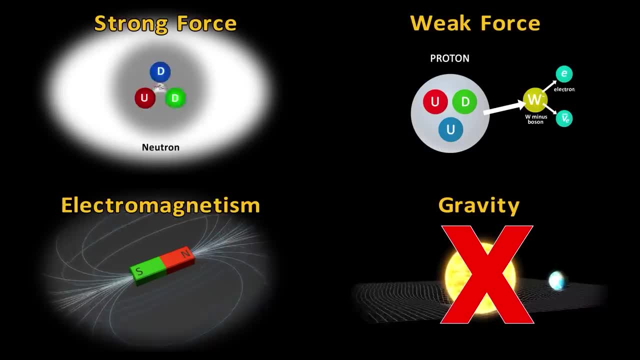 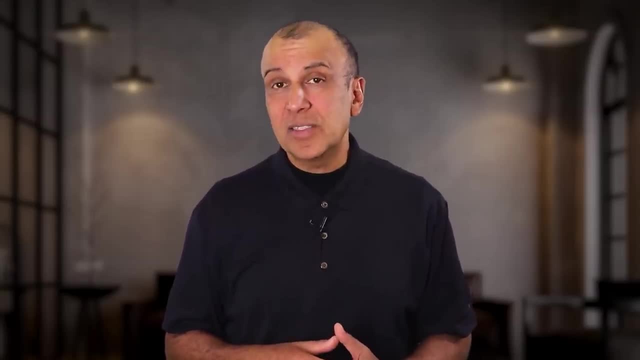 Gravity does not fit in the quantum mechanical model. Why is gravity so different And are we so sure that this is what reality really is? Why can't gravity be modeled by quantum mechanics? Let's examine this and find some answers coming up right now. 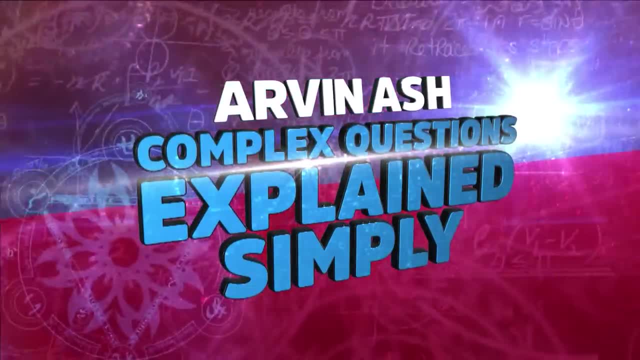 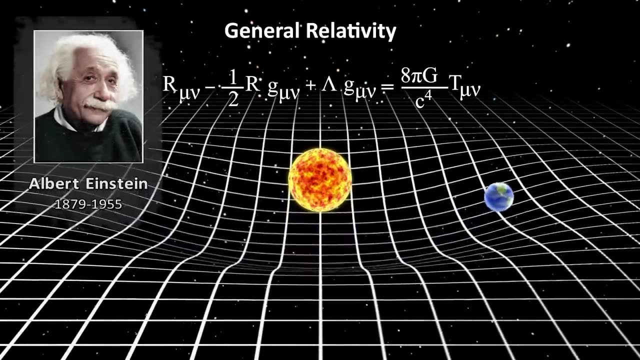 Today's topic is about the relativity of gravity. The best theory we have of gravity is the general theory of relativity by Einstein, and it's been proven to be correct in test after test for the past one hundred years. But it's still a classical theory, not quantum. 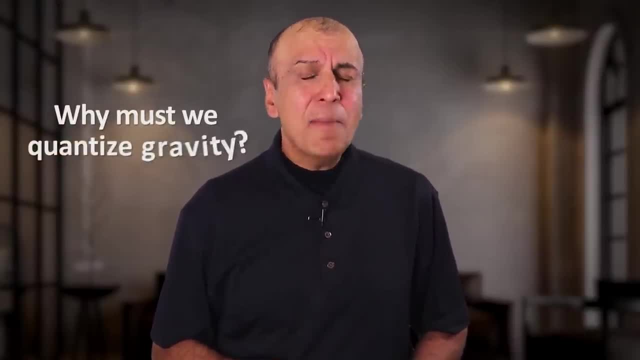 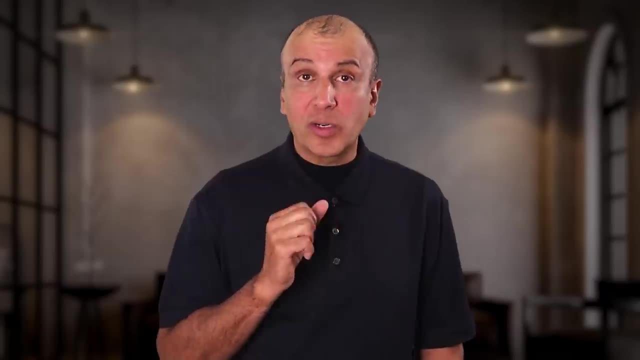 So why can't we leave well enough alone? Why must we quantize gravity? Let me give you a very simple answer: Because quantum mechanics works. It makes predictions And the predictions fit with observable data, in some cases to one part in one billion. 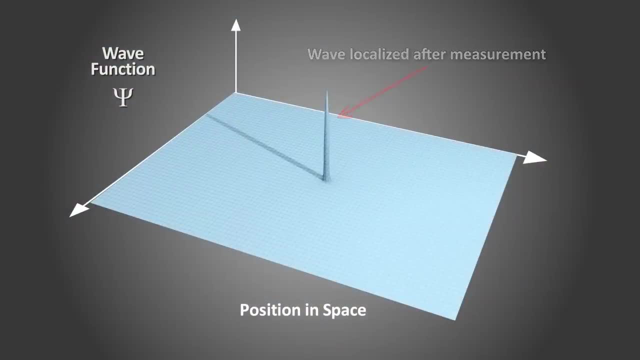 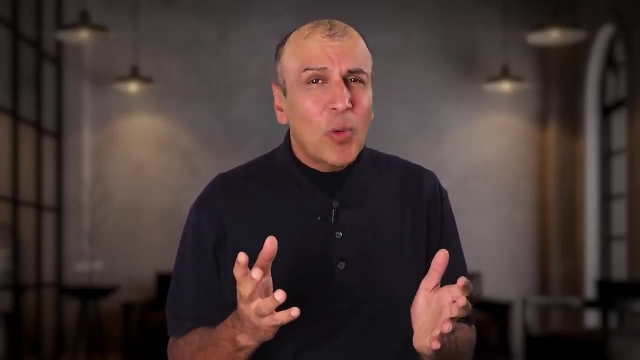 It's the most accurate theory of reality we have ever had. Now you may say: well, you just said that general relativity has been proven correct in test after test for a hundred years. Yes, that's true, Mostly, You see, general relativity falls apart at quantum scales, For example. 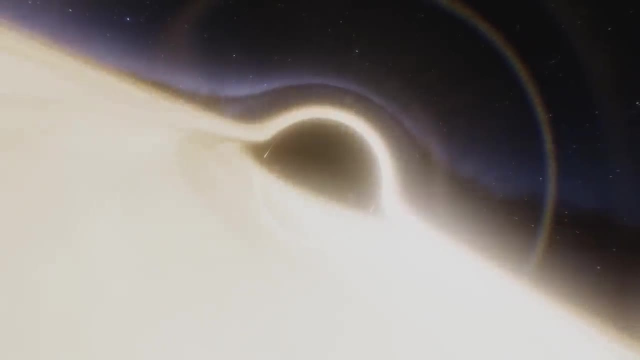 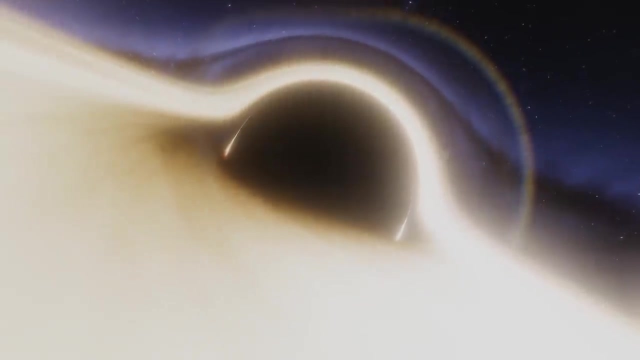 it cannot describe the singularity inside a black hole, where gravity theoretically becomes infinitely large at an infinitesimally small scale, or the presumed singularity at the big bang. These singularities are where quantum mechanics, the theory of the very small, 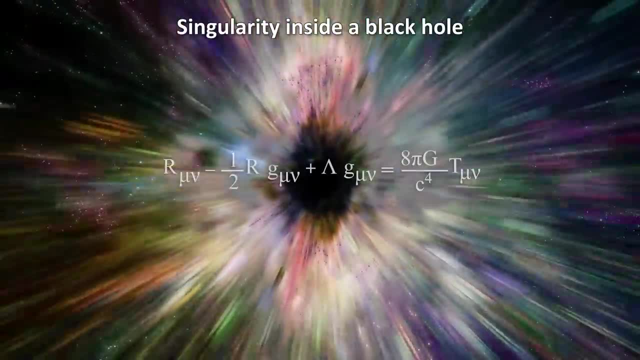 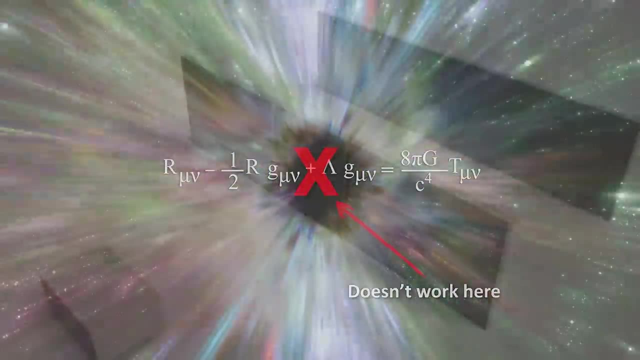 meets gravity. the theory of the very large, The equations of general relativity break down here, because it cannot describe how gravity works on quantum scales. Another example of this incompatibility is in the double slit experiment. This is a test on quantum mechanics, where 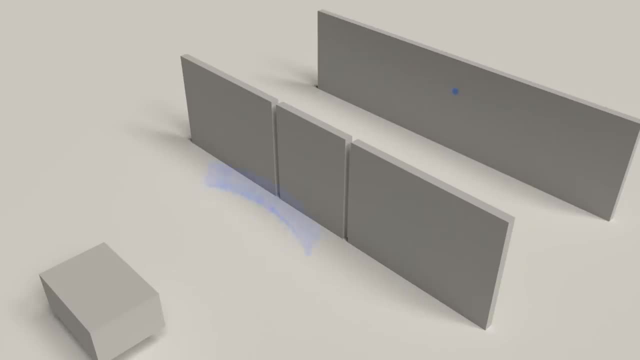 single photons or a lot of photons, or electrons or whatever they are. electrons are fired one at a time through a double slit. They show up as individual photons on a detection screen behind the slits. This looks fine for a while, but when thousands? 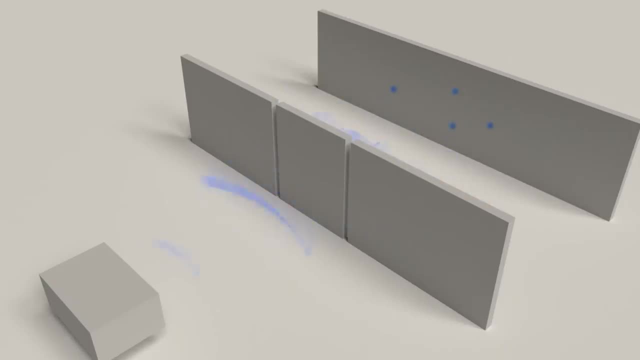 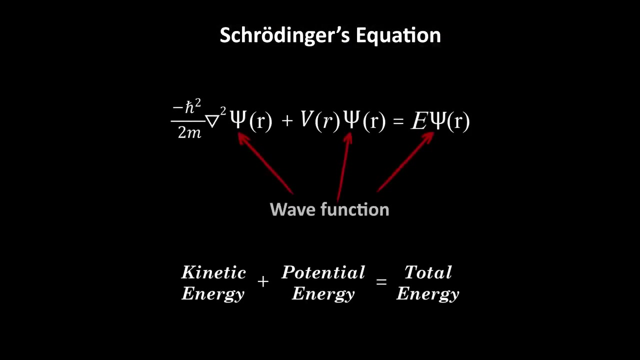 of these individual particles are fired, one at a time, over a long period of time, an interference pattern develops. It's as if the particles are waves. This is the classic test demonstrating the wave-particle duality of nature. The equations of quantum mechanics predict this behavior. 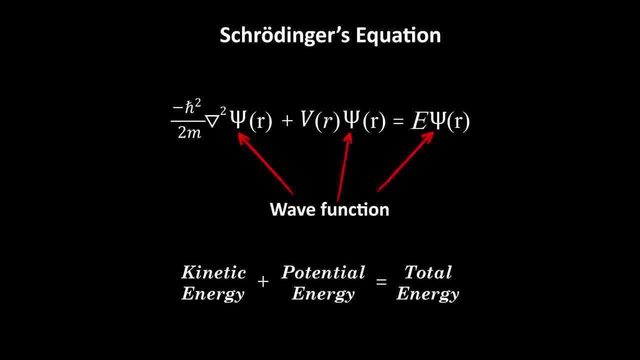 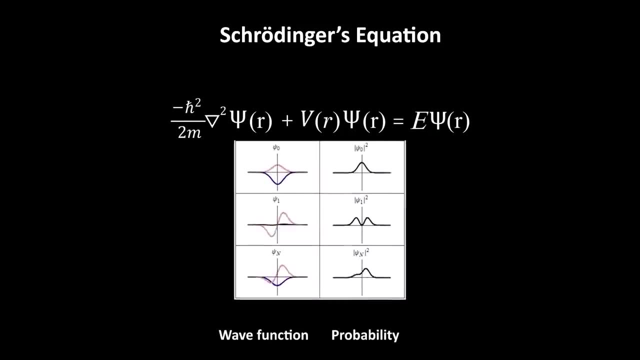 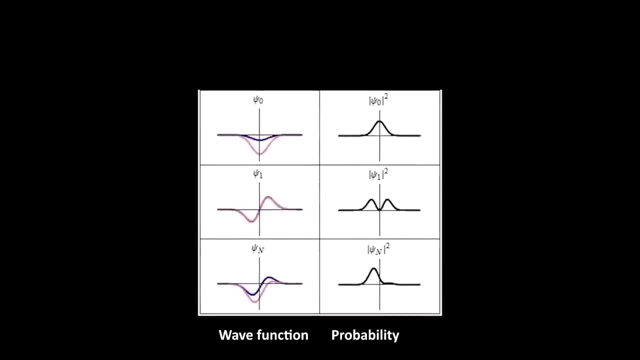 because they show that these particles are not like little cannonballs but are like a wave described by a wave function, And the wave function tells us the probability of finding these particles on any particular part of the screen. They tell us that particles are waves until some kind of interaction occurs, at which point the wave becomes localized. 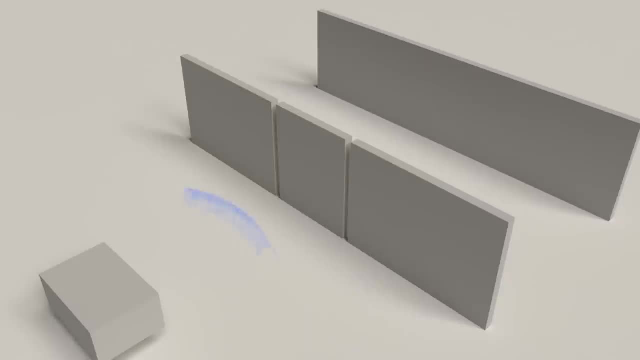 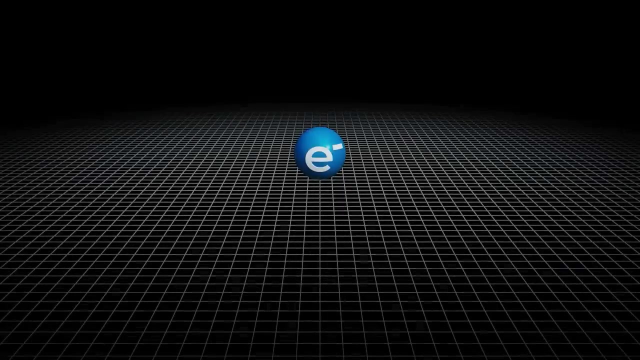 like a particle. In the case of the double slit experiment, the interaction of the photon or electron wave occurs in the form of a wave. The wave is a point-like wave which we perceive as an individual particle. But a photon or electron, just like any quantum particle, must also have a gravitational effect General. 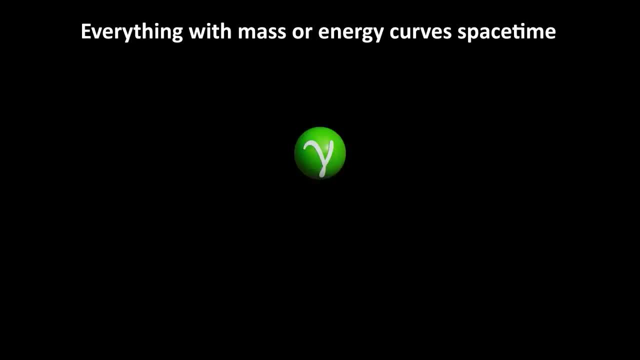 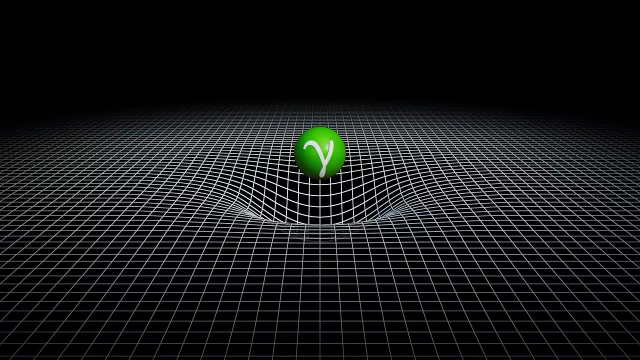 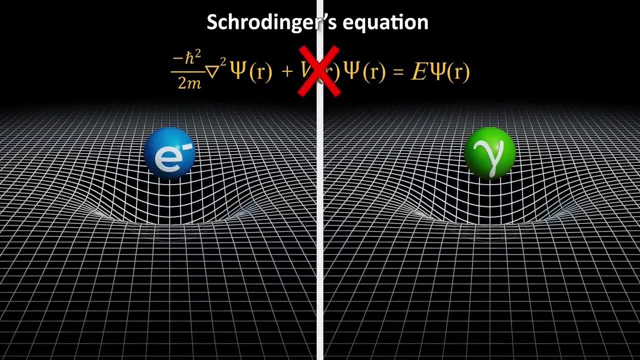 relativity tells us that anything with energy or mass affects the curvature of spacetime. This is what gravity is: the curvature of the background spacetime in which all matter resides and moves. But general relativity does not tell us how this gravity behavior behaves with a quantum wave function. If a photon or electron or any other particle 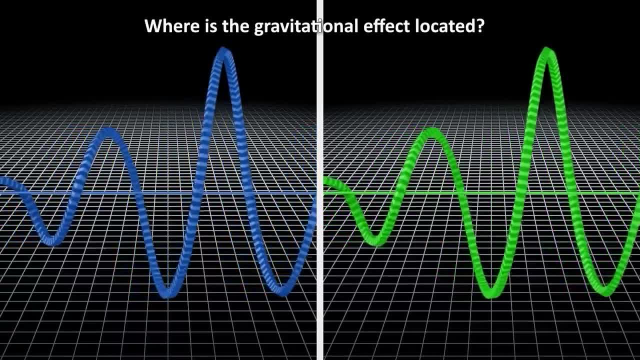 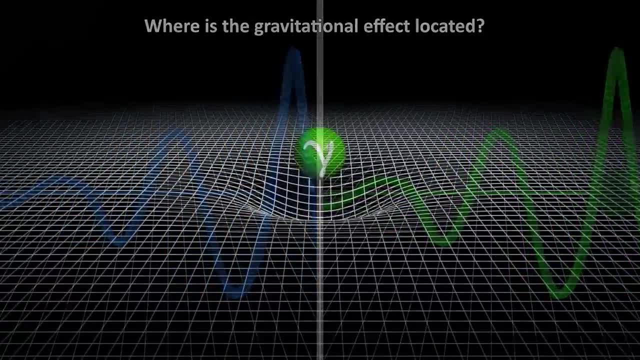 is a wave prior to an interaction, that is, it could be anywhere until the moment we measure it. where is its gravitational effect located? General relativity does not tell us how gravity can behave like a wave function. There is no wave function for gravity. The wave-like. 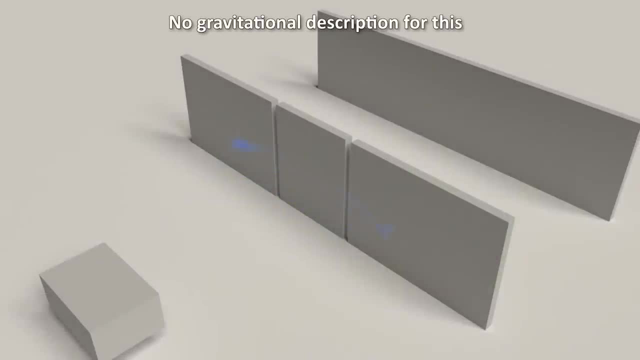 description of the particle prior to it hitting the screen does not have a corresponding gravitational description in general relativity. Yet since the particle has mass and or energy, it must affect spacetime and thus influence gravity. But we don't know how this works because we don't have a quantum description. 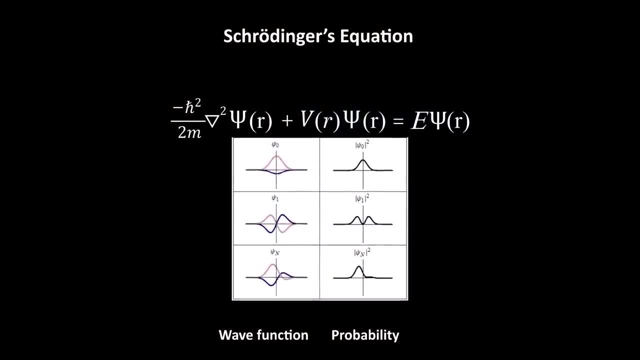 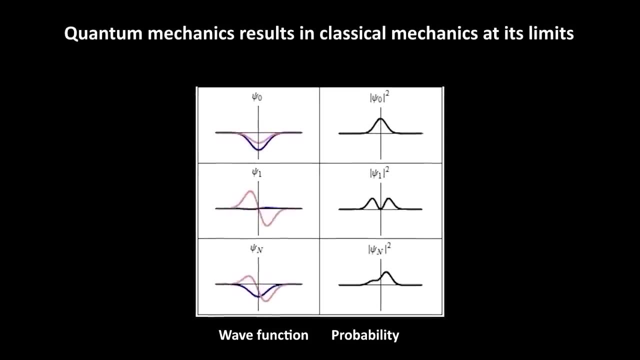 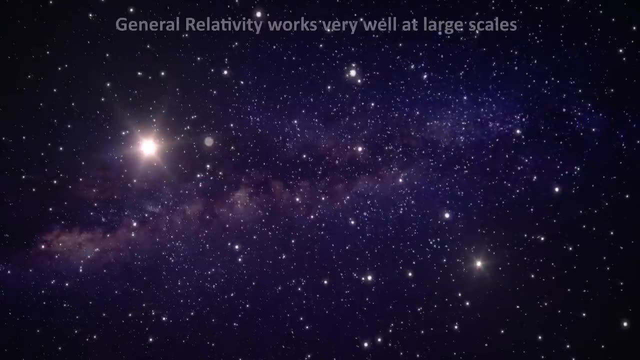 of gravity. So the bottom line is that we know quantum mechanics works And it works very well at the smallest scales, And it can be shown that quantum mechanics at its limits results in classical mechanics on large scales. On the other hand, we know that general relativity 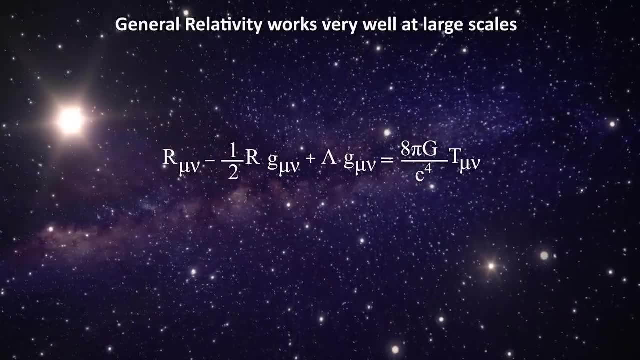 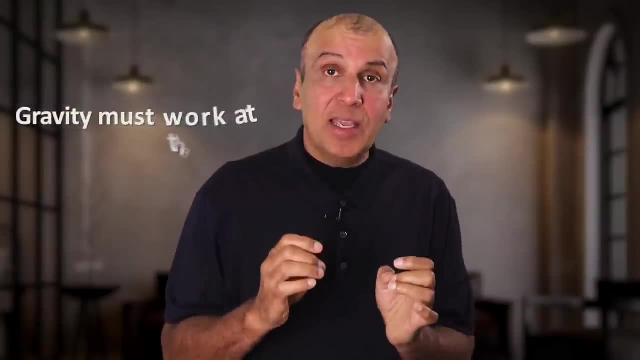 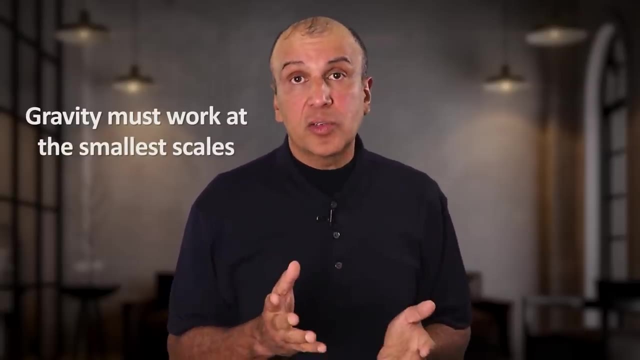 works very well at large scales. but the problem is general relativity does not work at all at the smallest scales. This simply cannot be, because gravity must work at the smallest scales, otherwise its cumulative effects would not work at large scales. This is why most physicists think general relativity must be brought into the fold of 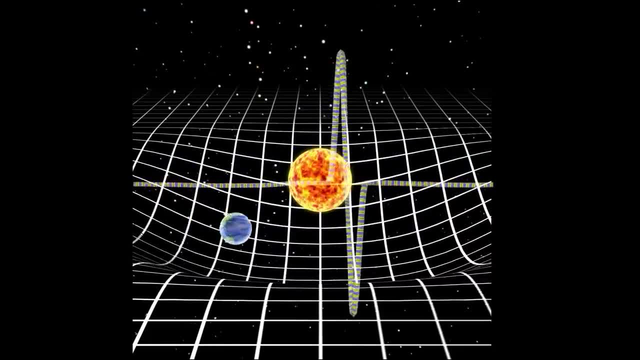 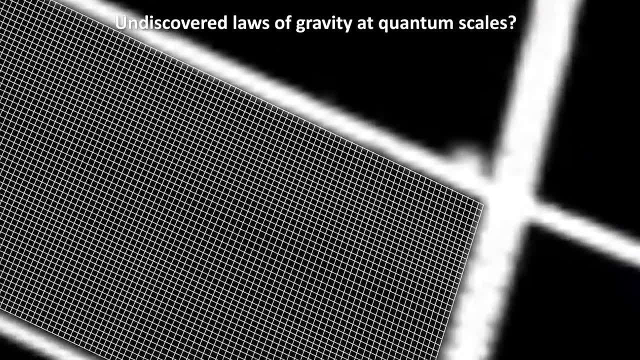 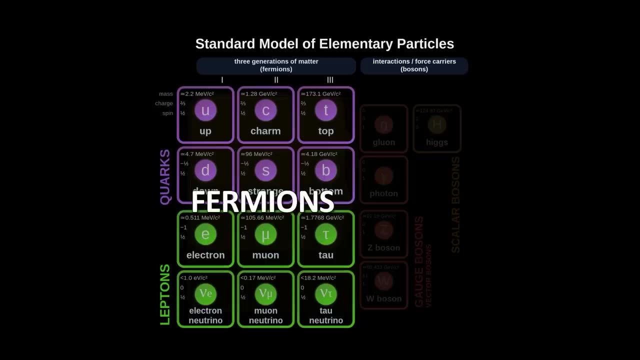 quantum mechanics. It is currently incomplete. It is highly accurate at macro scales but be described by as yet undiscovered laws at quantum scales. The problem is this: in quantum mechanics we have matter- particles called fermions- and force particles called bosons. 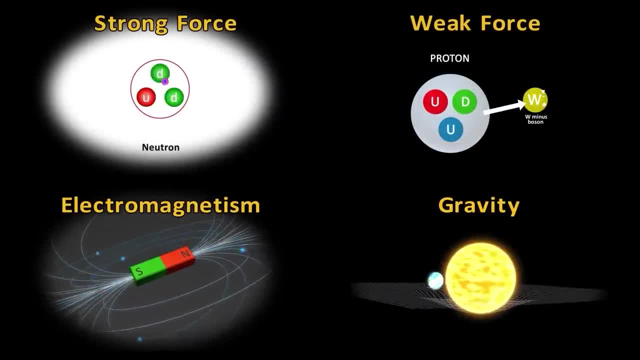 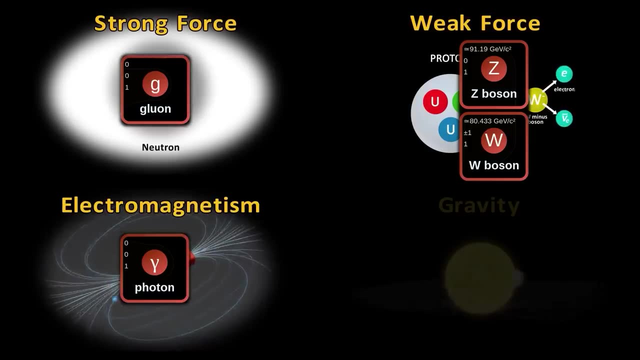 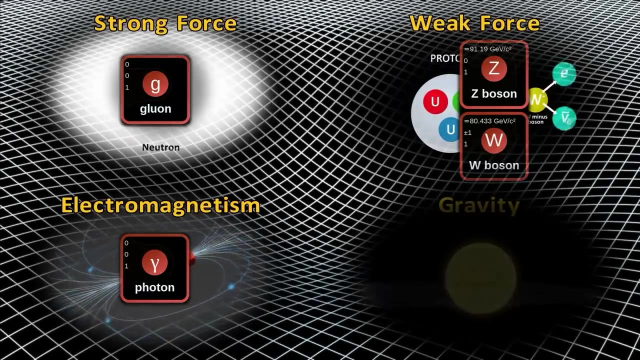 All interactions between matter particles are mediated by these force particles. In other words, these bosons of the standard model are responsible for the three forces – electromagnetism, the strong force and the weak force. And all these interactions happen with space and time as the background. 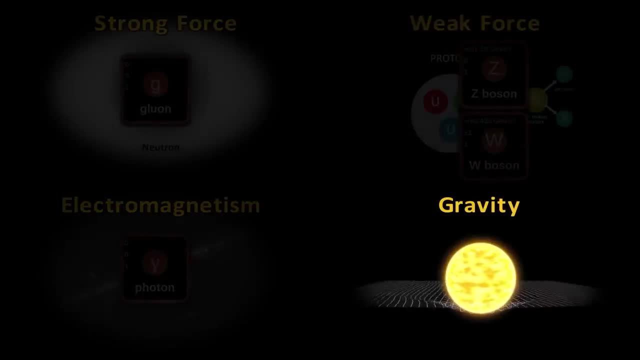 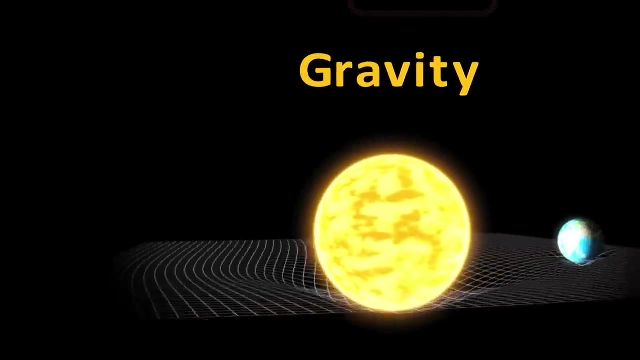 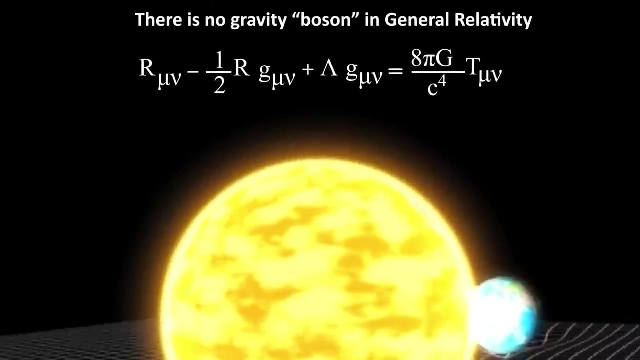 Gravity doesn't fit this picture because, as described by general relativity, gravity is not a force. Gravity in general relativity is due to a disturbance or a warping or a curving of the background space-time itself. There is no force carrying particle in general relativity, which mediates gravity between. 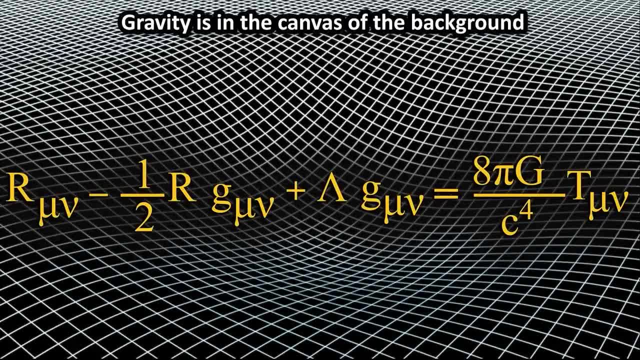 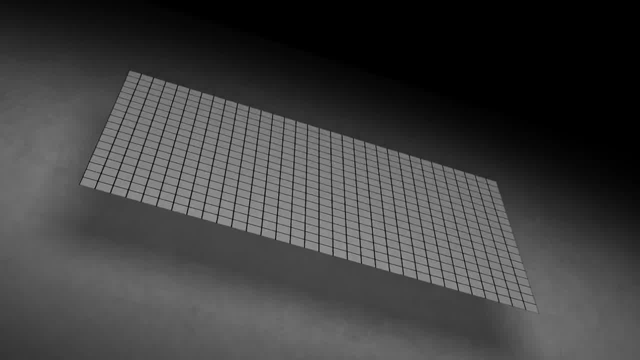 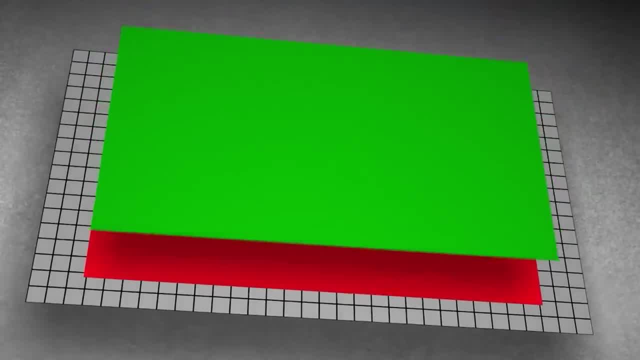 matter, particles, Gravity is embedded with space Within the fabric or canvas of the background in which matter and energy resides. This is much different than the picture we have of the quantum mechanical world, which can be thought of as the layers of paint on top of the background canvas. 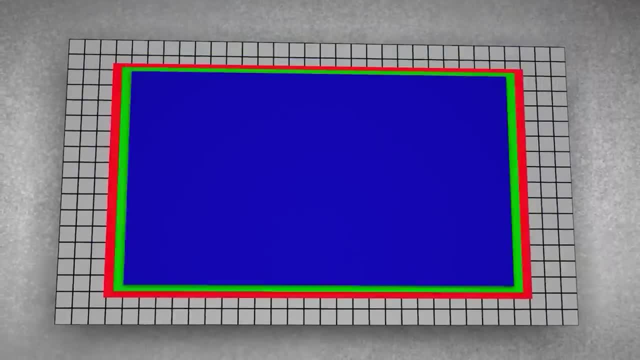 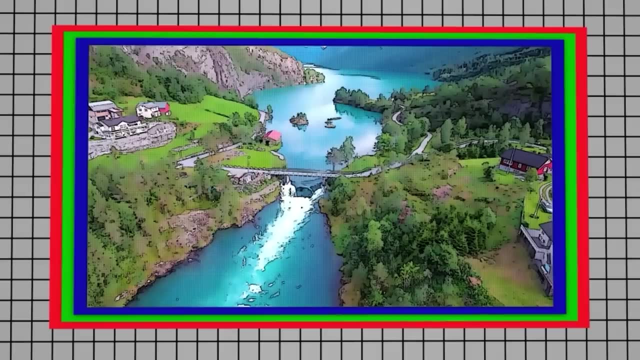 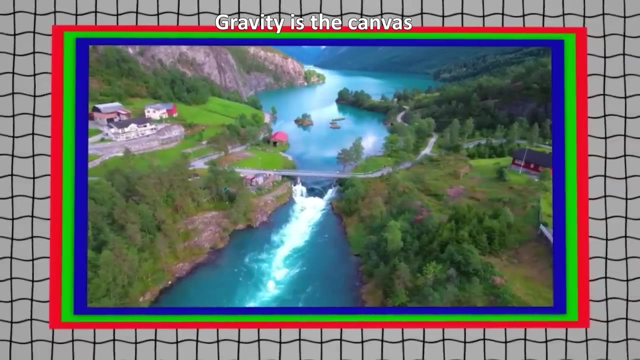 The waves of matter, particles would be like the different paint colors, and the interactions of these paint colors would create a beautiful painting, a painting that represents our beautiful universe, But gravity is the canvas itself. Gravity is the canvas itself And it is not an unmoving background monolith, like it is in a typical painting. 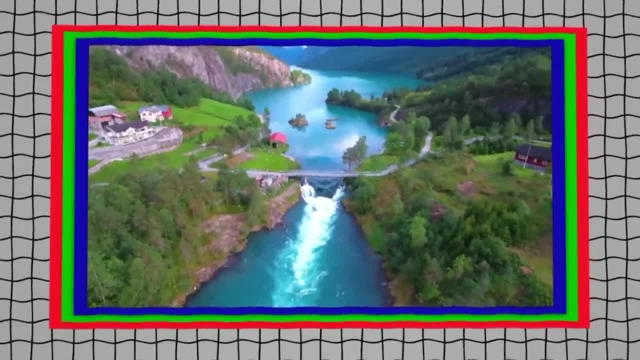 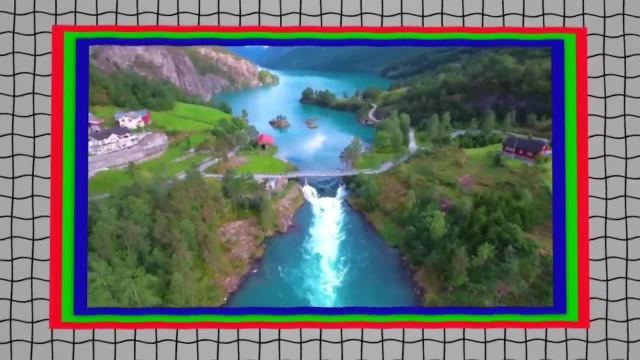 It is undulating, warping and curving such that it affects the overall look of the painting, which is analogous to how gravity affects our universe. Now, I want to point out that, just because general relativity as we understand it today, 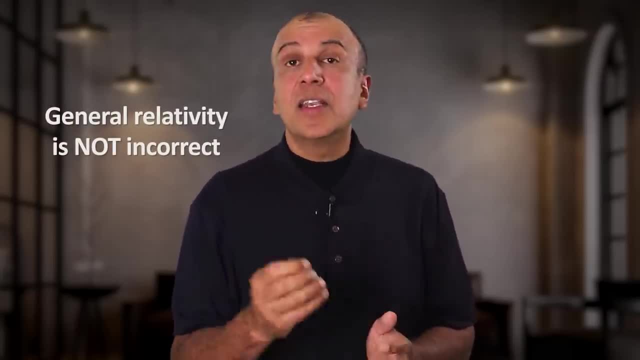 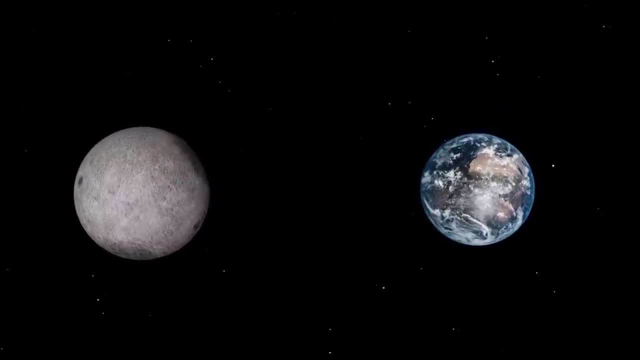 does not fit with quantum mechanics. it does not mean that it is incorrect. It is not incorrect, It is just incomplete. This is similar to the way that Isaac Newton's laws of gravity are not incorrect simply because Albert Einstein found a more fundamental theory. 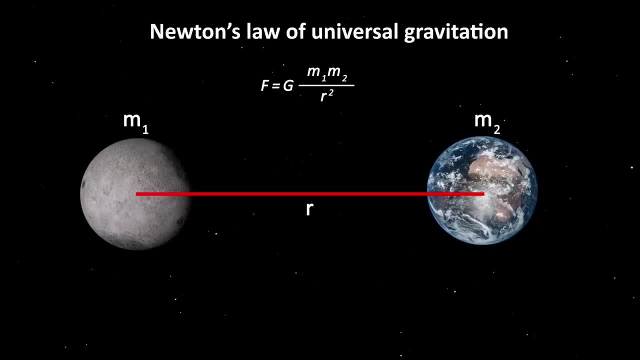 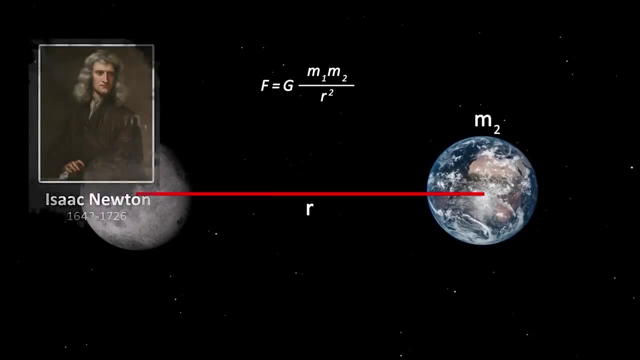 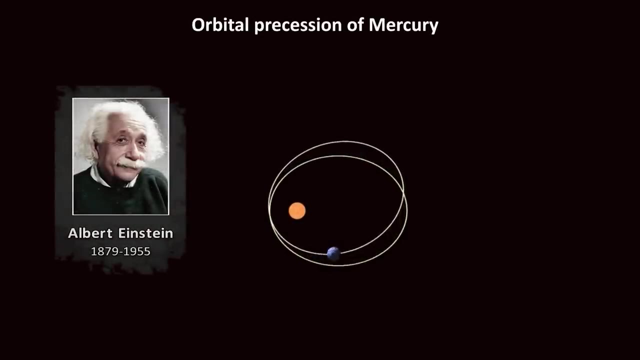 In fact, Newton's laws were used to send people to the moon. General relativity shows that Newton's laws are correct within limits. Only when Newton's laws don't work at extremely high levels of gravity, such as very close to the sun or near black holes, does general relativity provide a more complete picture. 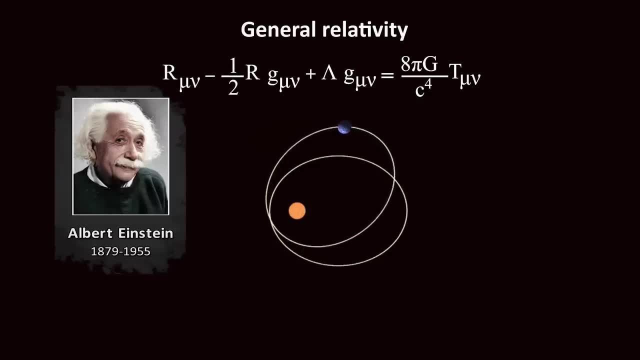 For example, General relativity does not work at extremely high levels of gravity, such as very close to the sun or near black holes. Does general relativity provide a more complete picture? described the precession of Mercury, but Newton's laws did not. Similarly, any quantum theory. 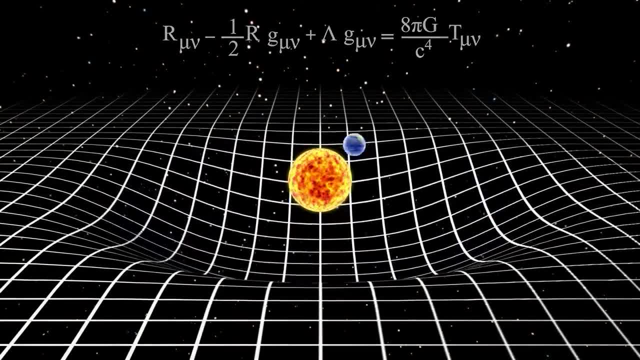 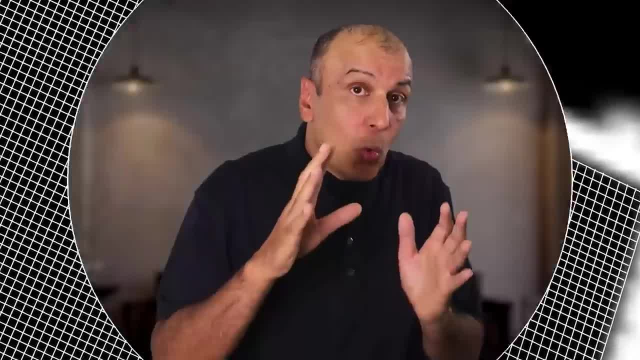 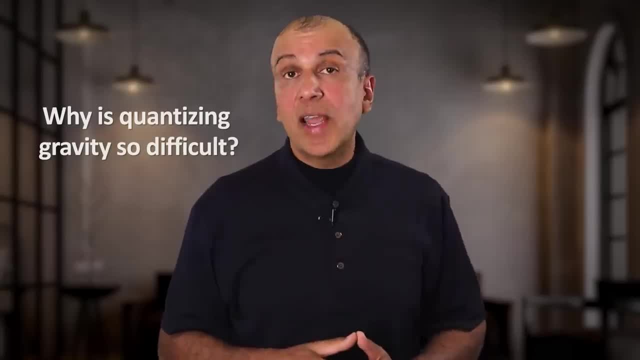 of gravity must show that general relativity is correct at its classical limits. It would just describe a more complete picture of gravity at quantum scales. So we don't have a quantum theory of gravity, even though this has been one of the most active areas of research for decades. Why is quantizing gravity so difficult? I am going. 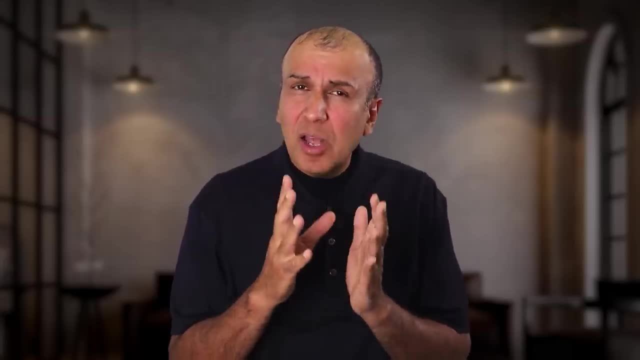 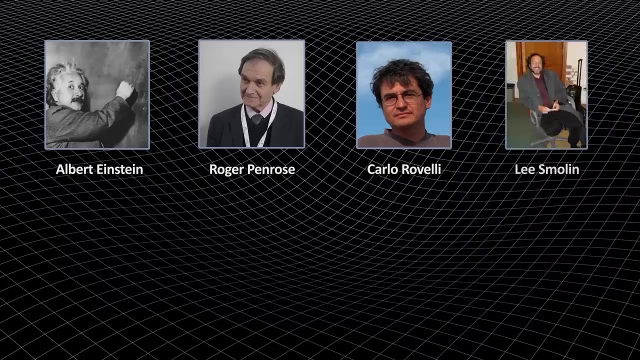 to explain this in the simplest way I can think of, but this is still a very difficult area to understand, so don't feel bad if you don't get it. with just one viewing, Some of the smartest physicists in the world couldn't figure this out, including Einstein. 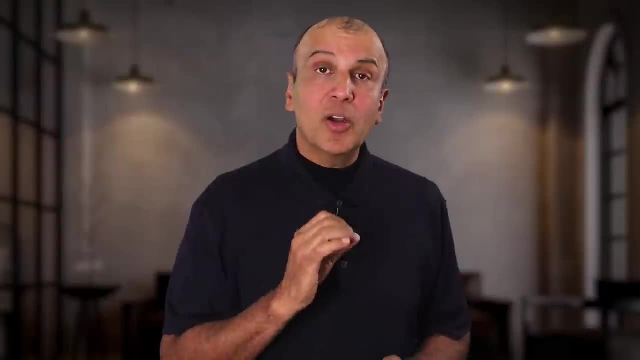 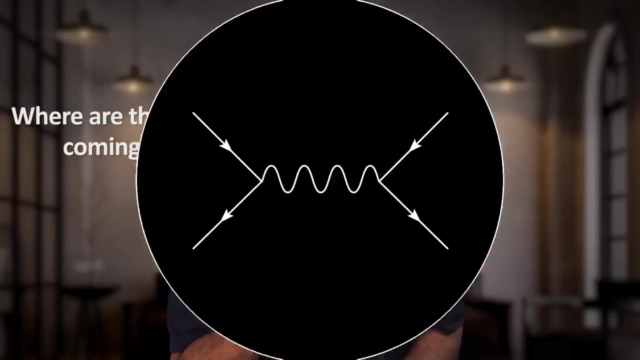 himself. Here's the basic problem. You've probably heard that infinities arise when physicists try to quantize gravity. Where are these infinities coming from? To explain this, let's use a Feynman diagram. This diagram represents an electron. 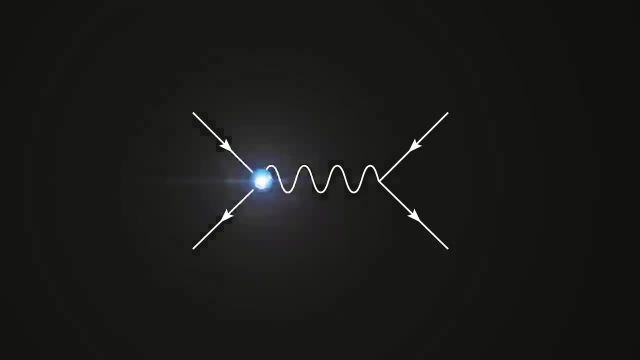 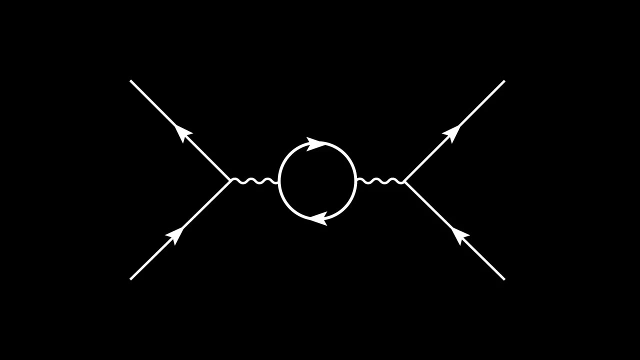 And a positron, Annihilating to create an energetic photon which then converts back to an electron and a positron. But quantum uncertainty is such that the photon in the middle, on its way to turning into an electron and positron, can convert to any one of a different. 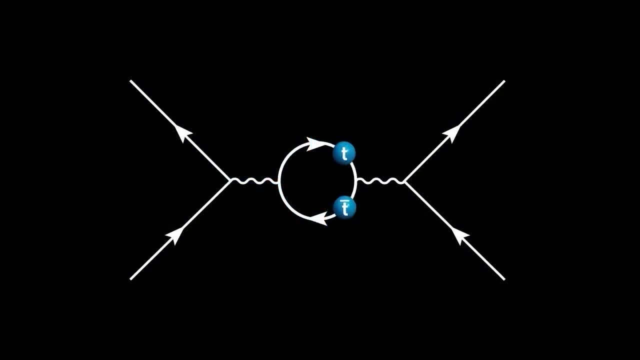 number of particles. For example, it can turn into a top core and an anti-top core which annihilates, Or it can turn into an electron and positron and back into a photon, Or it can turn into a muon particle bottom core, even a W particle on its way to becoming 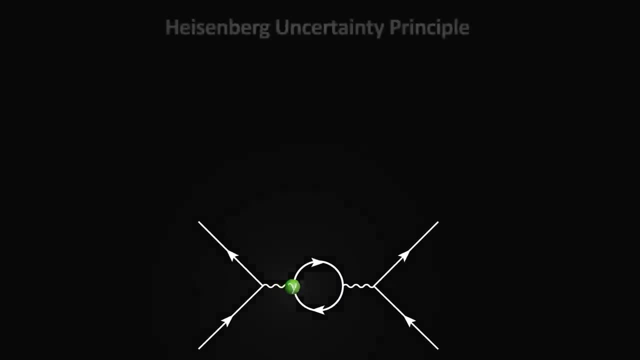 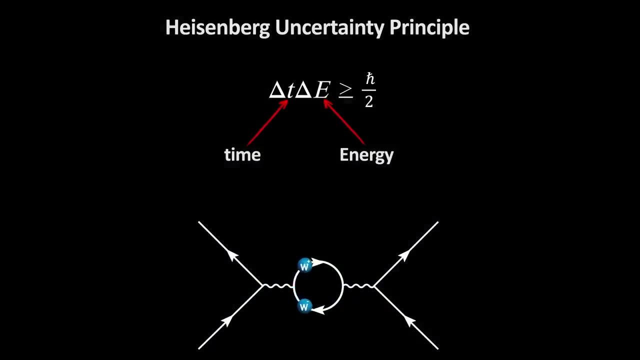 an electron and positron. It can do this because the uncertainty principle allows creation and annihilation of virtual particles. This means that particles can be created by borrowing energy from the vacuum of space for a very short period of time, as long as that energy 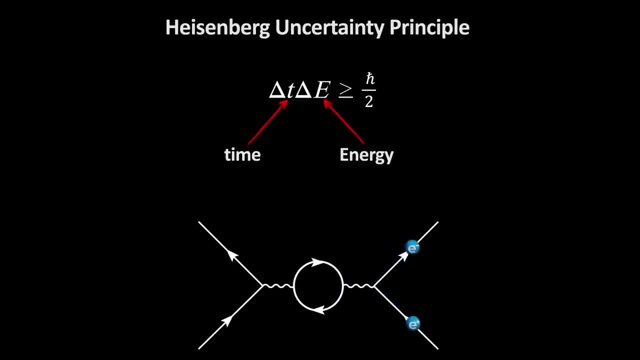 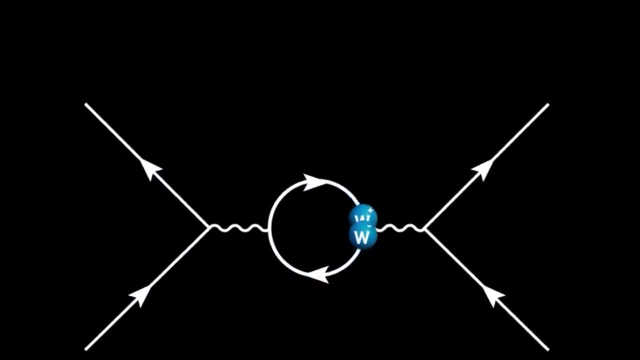 is put right back to the vacuum almost immediately. Since matter and energy are interchangeable, the energy can be in the form of just about any fundamental particle, And it can do this ten times, a hundred times, a thousand times, actually an infinite number. 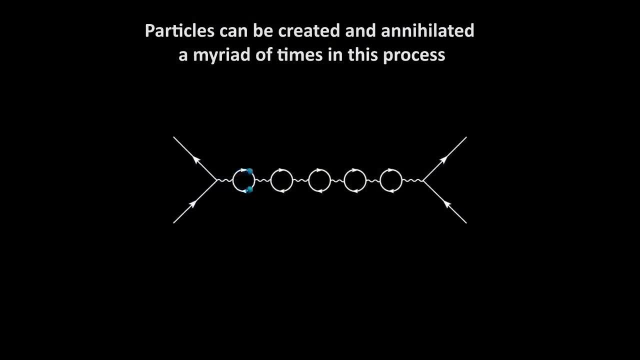 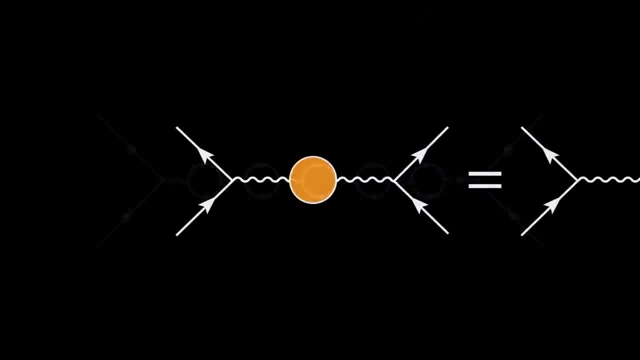 of times before turning into an electron and positron again. In other words, it can turn into a myriad of particles and it can do this a myriad of times. When describing this mathematically, we have to take all the momentums of all the particles and all potential interactions between: 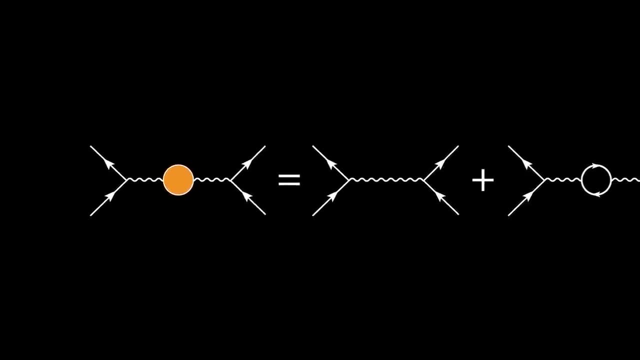 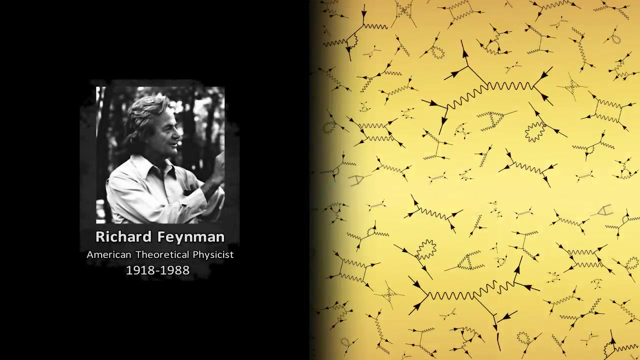 the various particles into account, There turns out to be an infinite number of combinations of interactions. This is where the infinities crop up in the equations of quantum mechanics. But a few brilliant scientists, most notably Richard Feynman, found a way to get rid of these infinities. 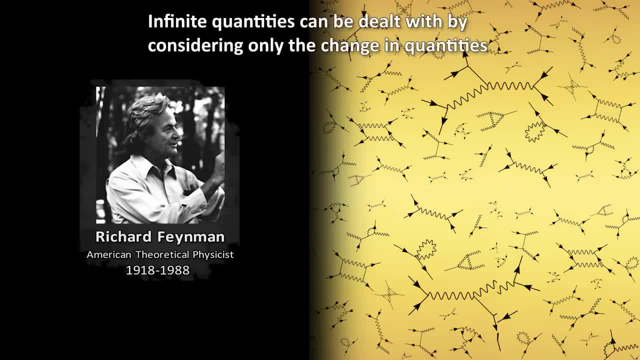 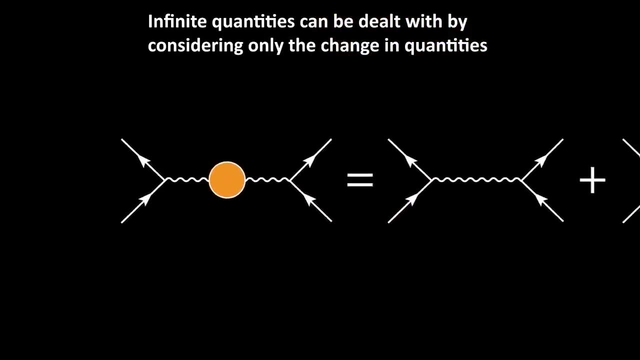 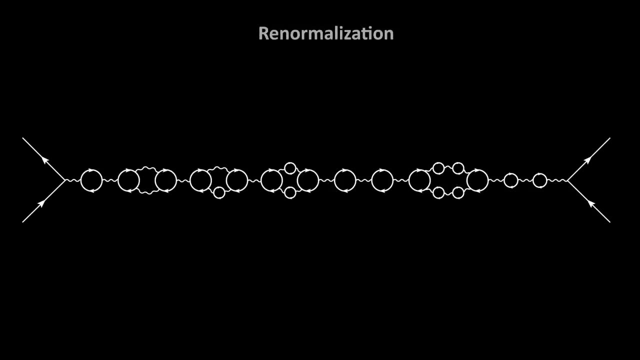 using clever mathematical tools, For example by showing that the infinite quantities themselves don't matter, but only how those quantities change. So even though the equations contain meaningless infinities, useful information can still be extracted from them. This process is called renormalization. 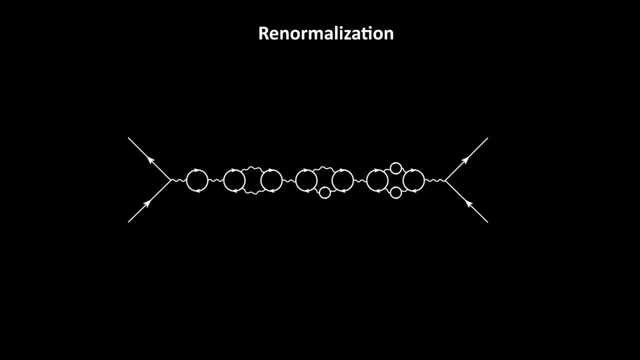 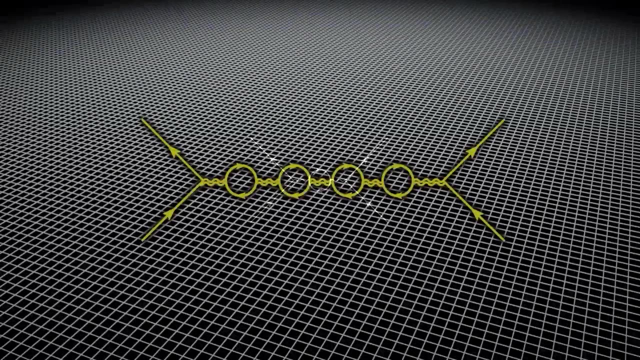 And voila, we have a quantum theory that works and the standard model is saved. But this renormalization process does not work when taking gravity into account. This is because gravity is not a force according to general relativity, as I said earlier. 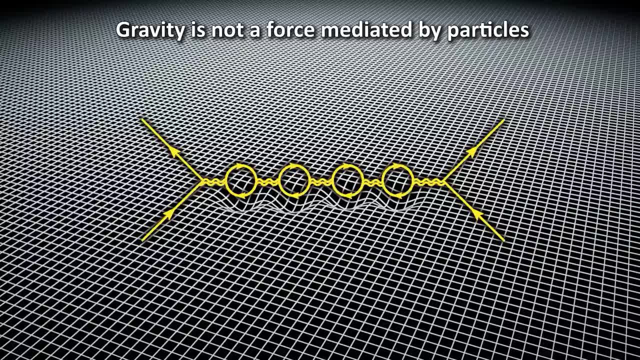 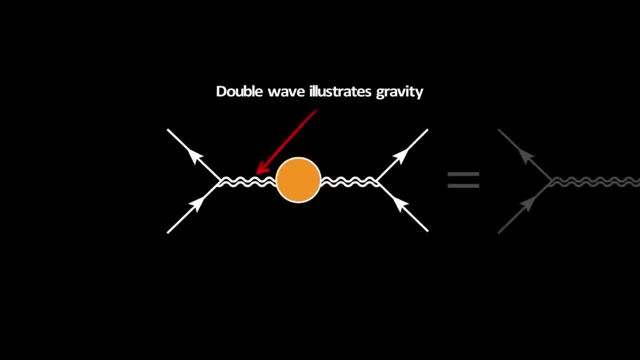 It is all about the curvature of spacetime. It is not about the particles, as is the case in quantum field theory. It is about the background on which these particles or fields reside. So you might understand the problem If we use the same Feynman diagrams as above, but now, instead of just the math representing 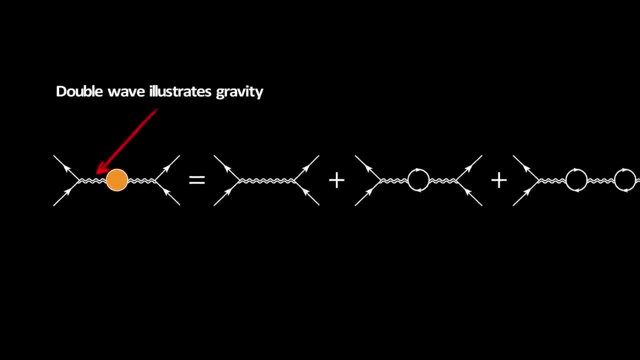 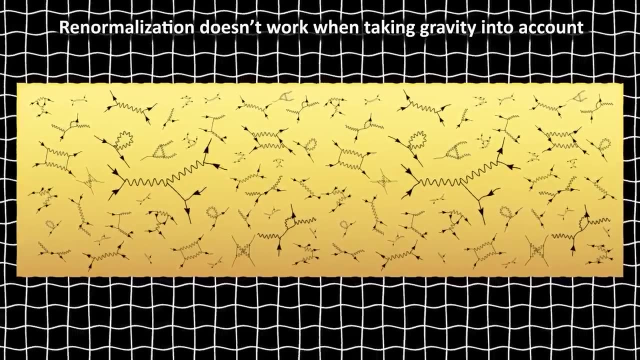 the myriad of particle interactions, we also have to take into account every possible configuration of spacetime underneath every one of those possible interactions. this makes it such that we now can't get rid of the infinities. The math can't be solved, So we are stuck. 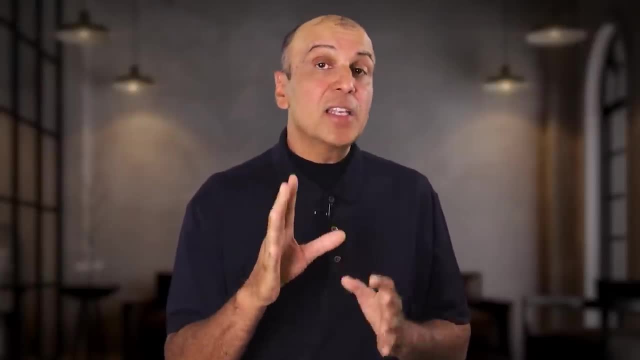 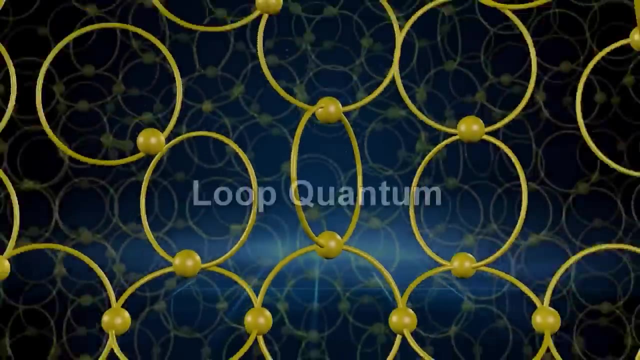 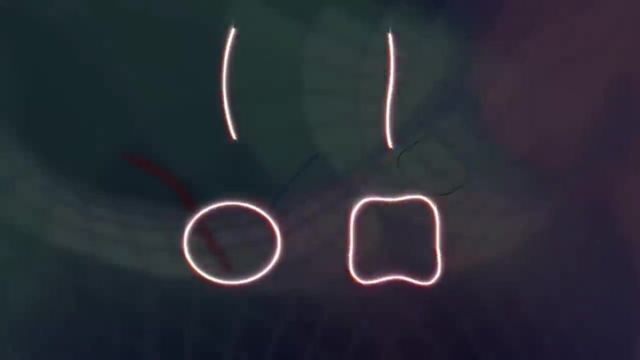 Now, just because we can't solve it does not mean that solutions don't exist. The only way to solve this problem is to use a completely new approach. Some valiant efforts have been made. Two of the most well-known attempts are loop, quantum gravity and string theory. I have a video on this if you want to learn more Basically. 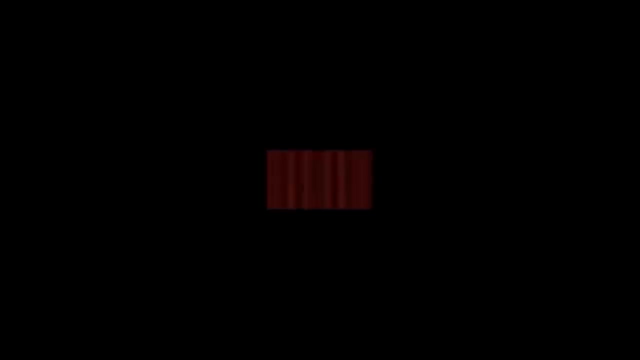 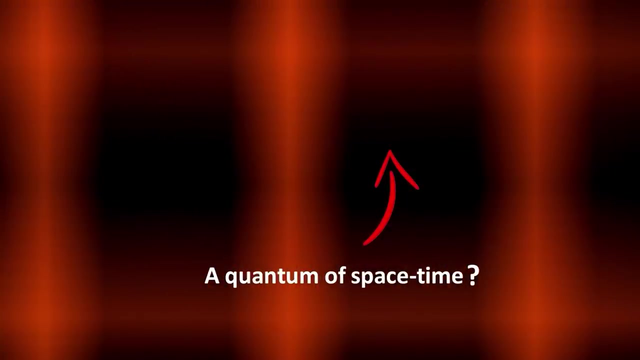 loop. quantum gravity attempts to quantize the background of spacetime itself. Describing reality is a pixelated landscape, somewhat like the pixels on your TV screen. So instead of finding a particle that mediates a gravitational force, it could be a particle that mediates 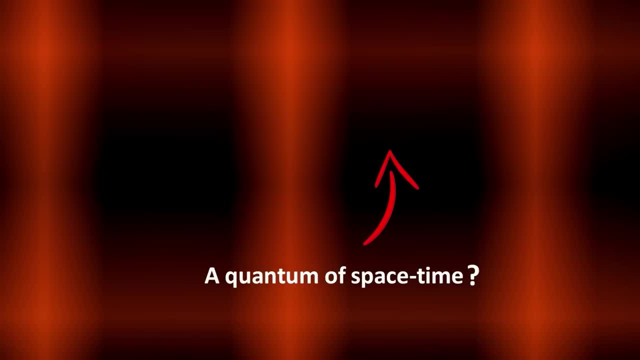 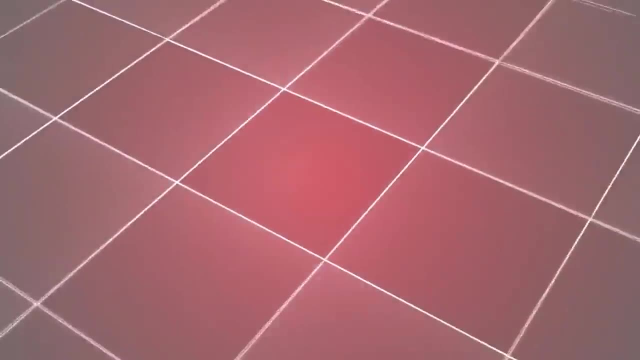 a gravitational force. So, instead of finding a particle that mediates a gravitational force, it could be a particle that quantizes the entire spacetime background itself. And string theory is an attempt to describe reality as a completely new paradigm where everything is a string vibrating in. 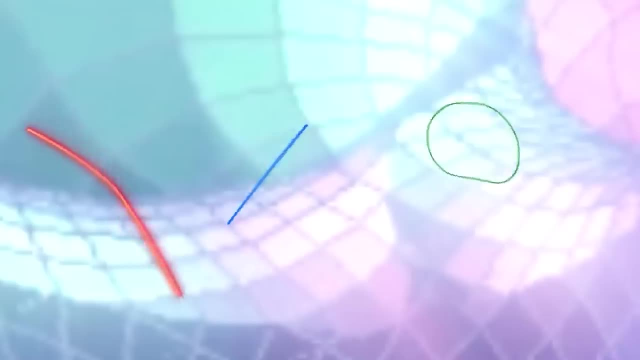 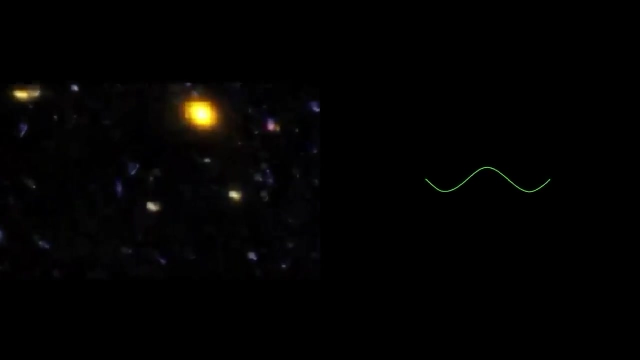 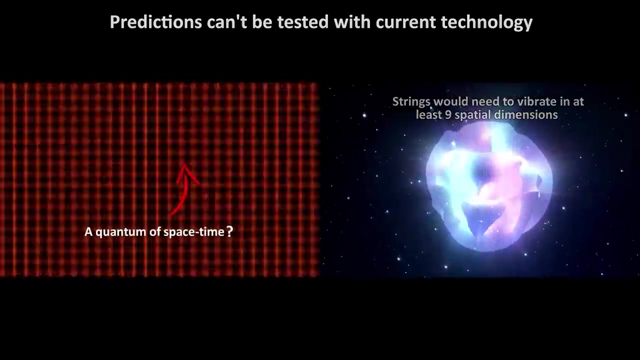 multiple, unseen small dimensions. It treats gravity as a force which is mediated by a new particle called a graviton. But the problem with both these theories so far is that they largely don't explain observed phenomena And they don't make any testable predictions. So we are still 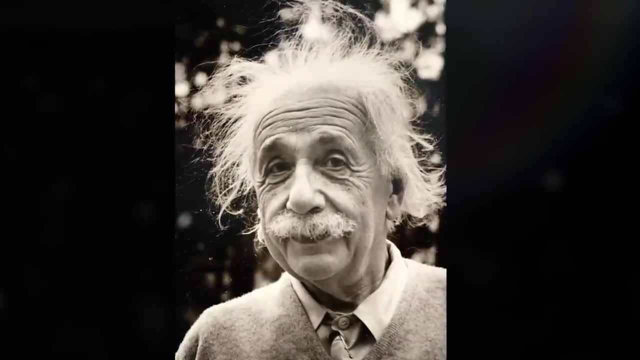 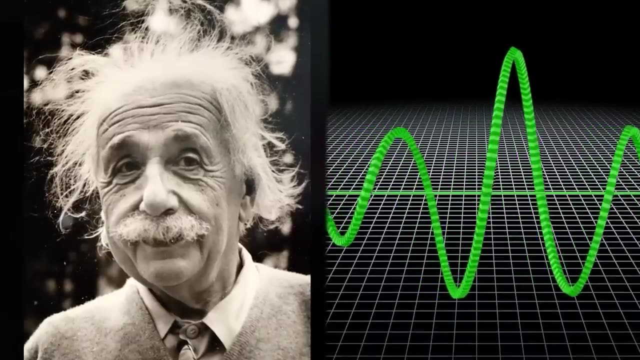 stuck. Even Einstein, until his last day on earth, had been attempting to solve this issue of reconciling gravity with quantum mechanics, but was unsuccessful. But in all likelihood there is a solution out there waiting to be discovered. It is probably going to take the 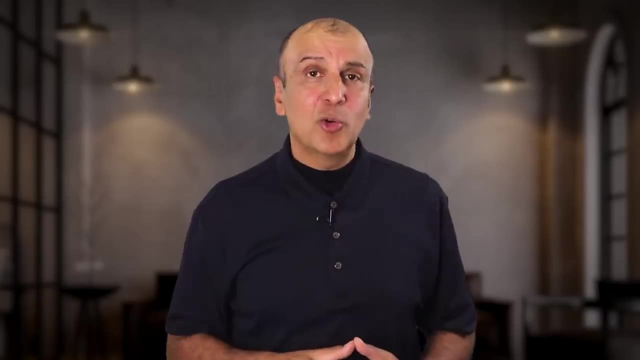 right individual with a bold and perhaps radical new approach viewing the real reality. And if you would like to learn more about the reality we live in, there is a wonderful course on Wondrium called Redefining Reality. The answer is in the description of this video. And if you would like to learn more about the reality we live in, there is a wonderful course on Wondrium called Redefining Reality. The answer is in the description of this video, And if you would like to learn more about the reality we live in, there is a wonderful